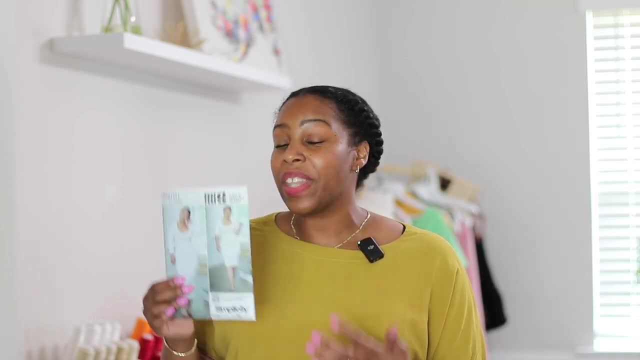 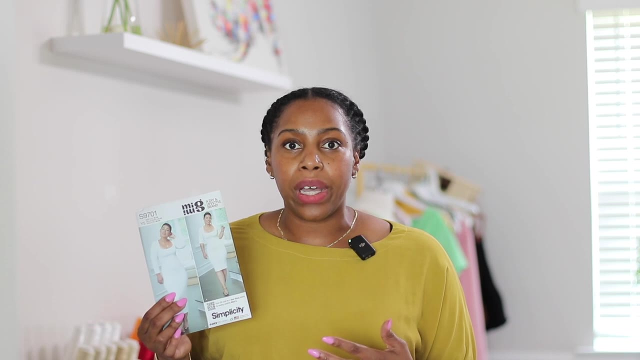 easy that you may prefer to start sewing with. I also like this because it comes with a sew-along video And that just helps with answering questions. So maybe you don't know what you're doing, If you don't know what reinforcing is, or if you don't know what stay stitching and 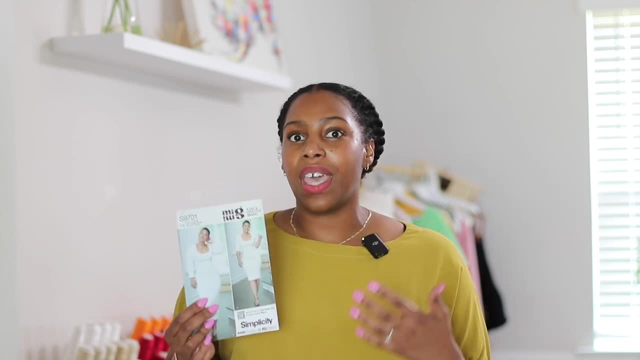 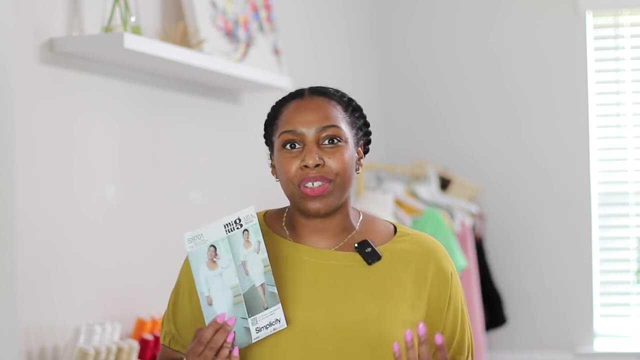 understitching is. that's all covered in the sew-along, So you'll kind of see like understitching, you can see it being done. That just helps you just get better with learning techniques as opposed to trying to learn them on your own. If someone is showing you how to do it, I'll take. 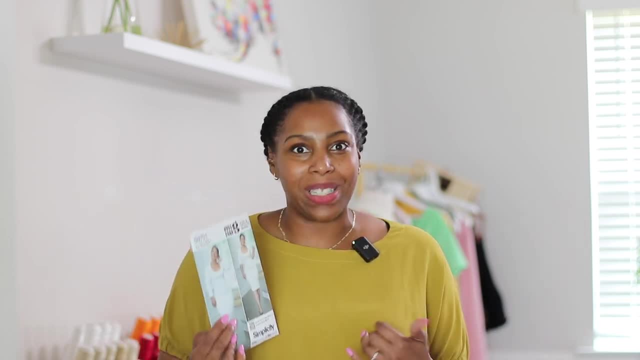 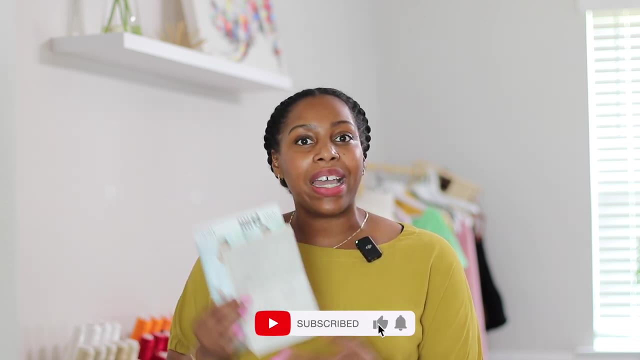 a visual any day. That's just me personally. But if you're going to show me, yes, that just helps me learn it faster. The last reason why I picked this one for this video is because it has five pattern pieces. That's a win. If you're starting out, you want something no more than five pattern. 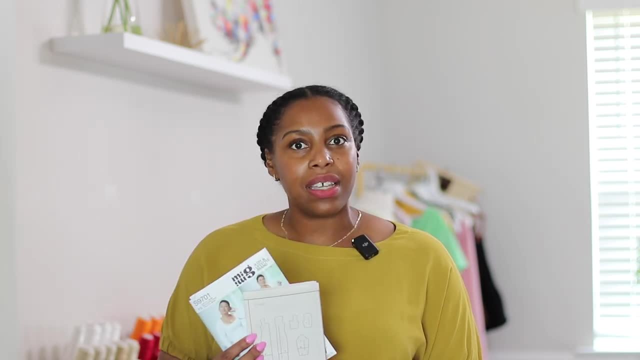 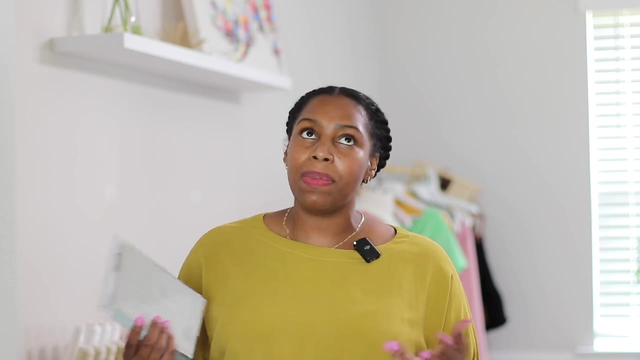 pieces. Anything over than that isn't really that easy. I mean maybe, but I wouldn't recommend that for a beginner or an advanced beginner- maybe advanced, but not so much If you still want to keep the pattern pieces low. I feel like when you're just starting out, you're learning, you. 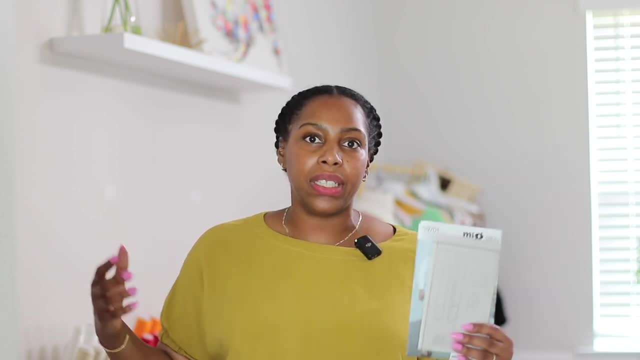 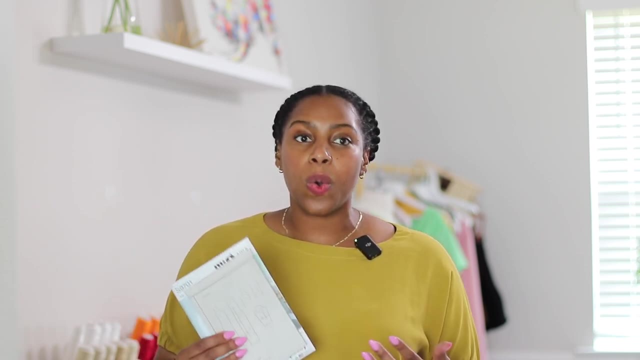 want to do stuff. I won't say quick and fast, but long, lengthy projects, I don't know. They can kind of mess with you a little bit, especially if you're not a hundred percent sure or if you're not confident in what you're doing. you don't want to discourage yourself by getting a pattern that. 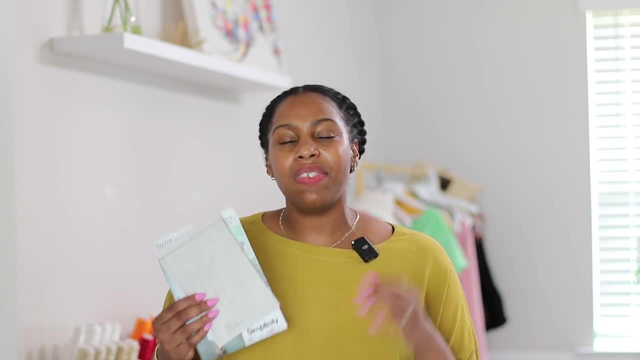 has a lot of pieces. even though they say it's easy, It's still even small. things like that can really mess up for people who are beginning to sew. if the pattern has 10 pieces but they didn't realize it was one, that was maybe three pieces that you know they can whip up and have that. 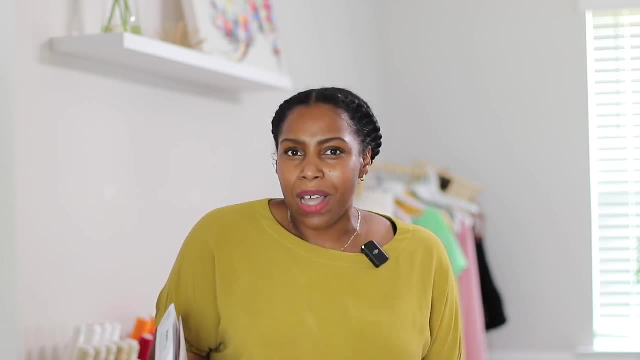 instant. um, you know that confidence boost Cause that's what it's all about. If you're just growing and getting better, you'll keep doing it. But if you're defeated from the gate, it's kind of hard, unless you really just absolutely love it and you're determined to do it. 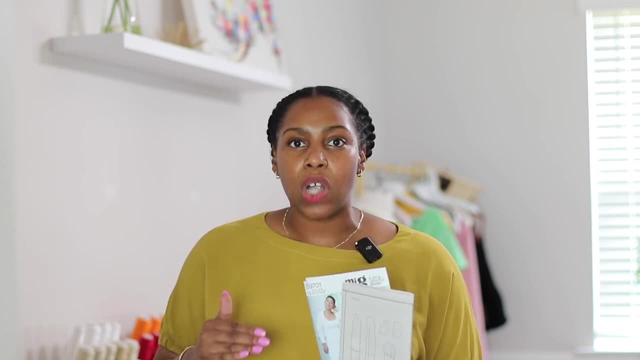 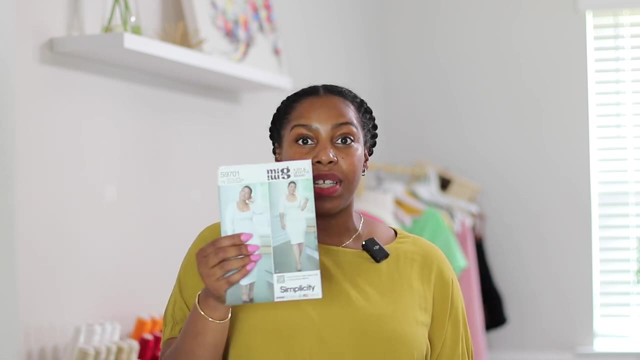 But that's what I would say about that. Look for patterns that have maybe five or under pattern pieces If you are in that beginner, advanced beginner sewing level. So again, simplicity: nine, seven, zero one. I do recommend this for an advanced beginner or someone that's ready to start. 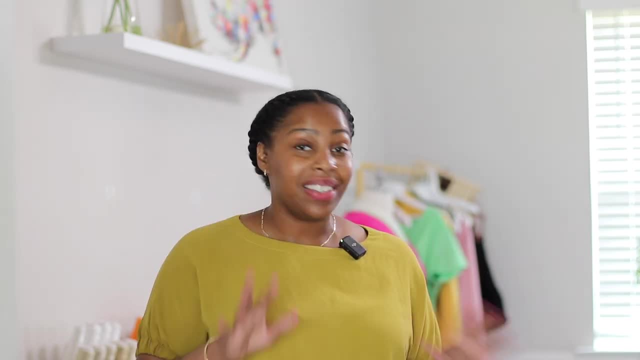 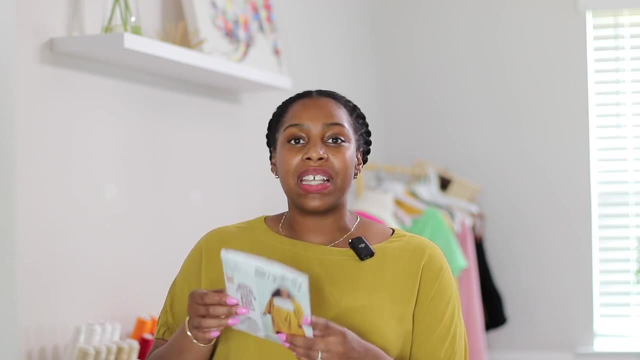 attaching linings and facings. This is a good one. The next pattern on my list is simplicity. nine seven, one seven. This is an easy to sew pattern. This one here is listed as easy- not very easy, but it's still in that easy category. You have a women's knit top. 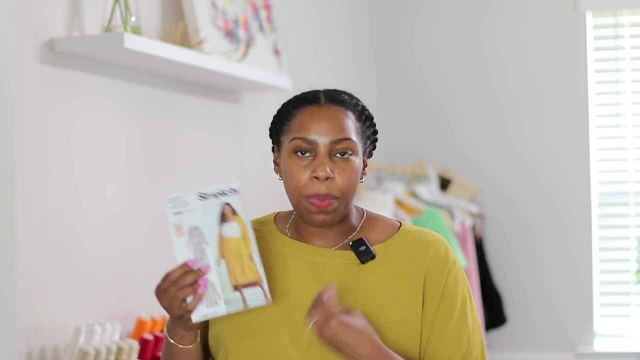 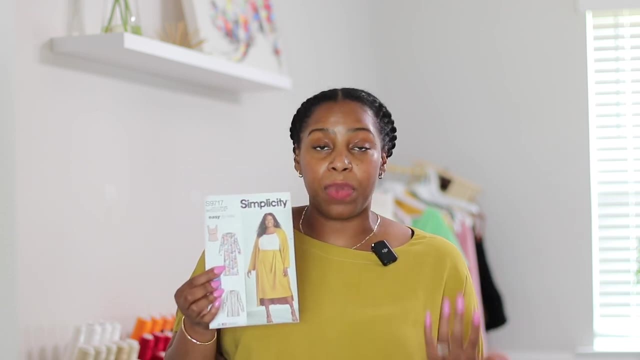 cardigan and skirt. So this is like a little wardrobe pattern here. You can pair these pieces together or make them and wear them as separates. This is just a really great pattern, I think, for beginners, because you can literally sew every piece on here And, like I said, have a whole. 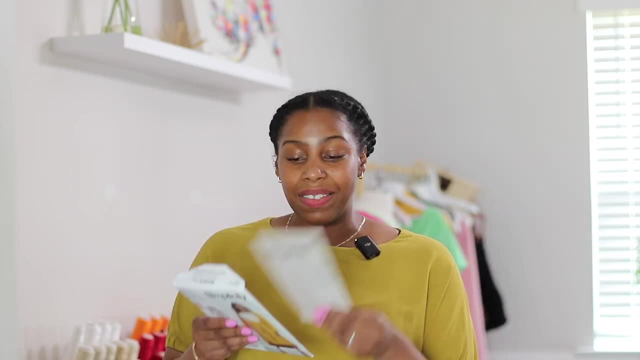 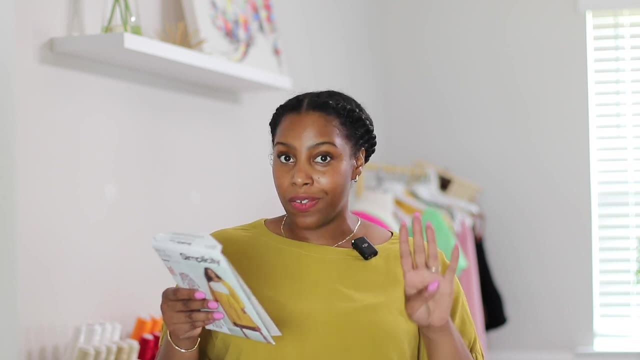 bunch of them separate, So this is a great one I think that you can start with. I have the guide sheet here. There's a total of 13 pattern pieces, but hear me out for view a, which is to tank, You only have four pattern pieces, So it still falls into that. you know, good beginner project. 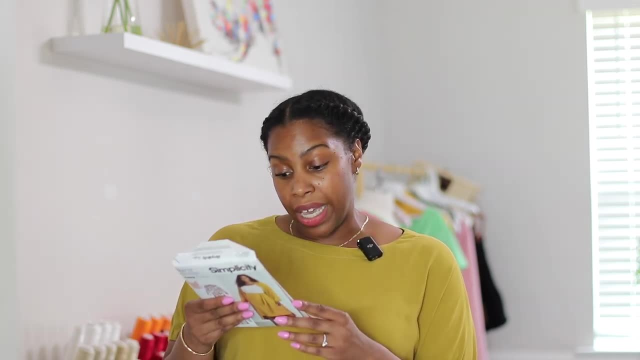 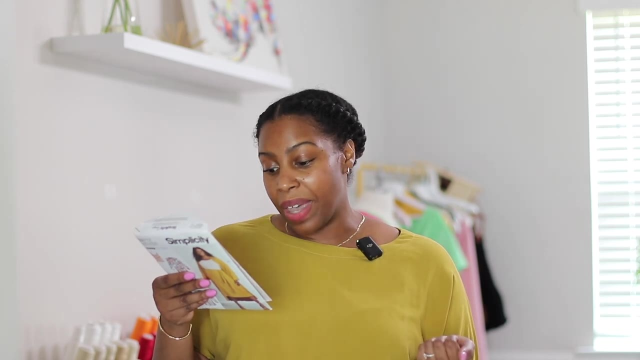 garment project. to start with, for the skirt, You have four pattern pieces: the front, the back, the waistband and the tie belt. for the cardigan, You have five. So each one of these pieces on this pattern. I again, I think it's going to be a little bit different. I think it's going to be a little bit. 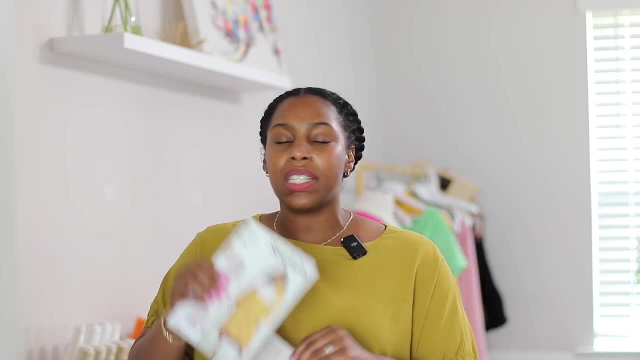 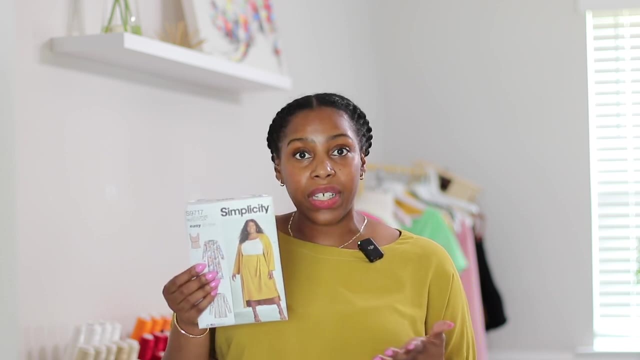 different for beginners because it's not a lot of pattern pieces. It's not 13 pieces for one, it's 13 pieces and you get three looks here. So I really do like this pattern. Like I said, it's very easy. It is knit fabric, So knit fabrics, depending on who you talk to, will say: 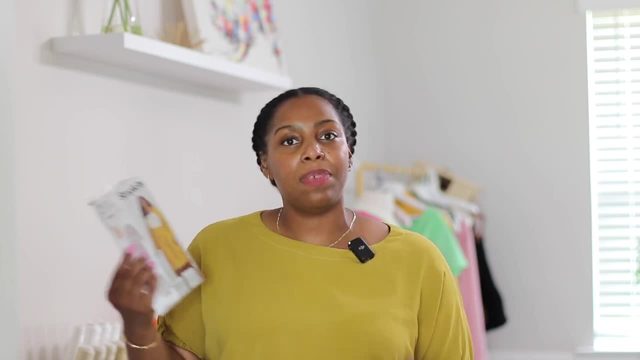 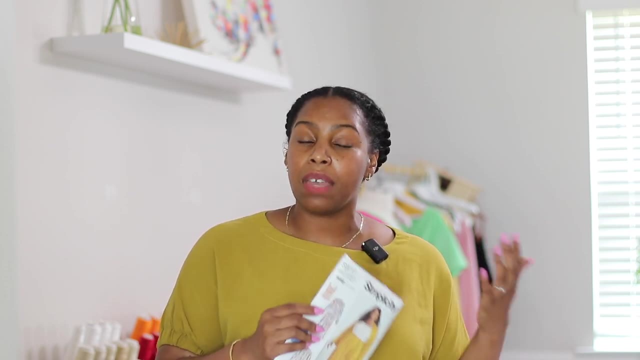 that it's a great fabric to start working with because, depending if you make a mistake or not, it may still fit, While, on the other hand, people may say, start out with wovens, because sometimes sewing with knits can be a little tricky if you're a beginner, So it's really a toss up. 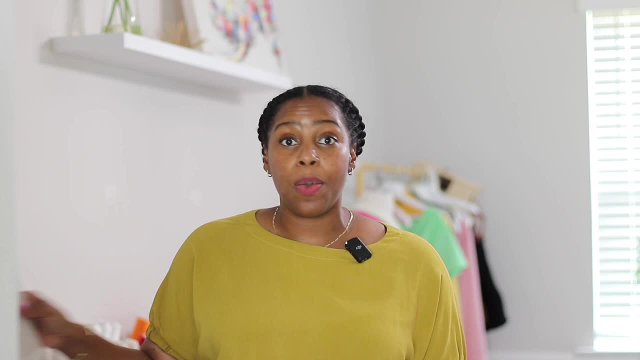 honestly, depending on, like I said, who you talk to, they may say: stay away from knits, but you may talk to someone else that say: start with knits. So, honestly, I recommend that you start with what you like. If you wear a lot of tanks and a lot of pull-on knit garments, 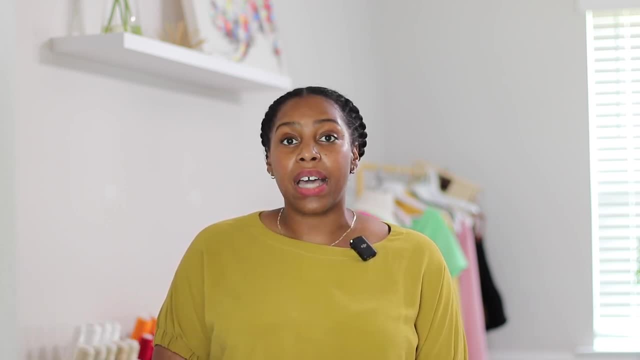 then start with the knit project. If you see yourself wearing a lot of- maybe just tops like this, maybe like boxy tees or maybe gathered skirt, start with the woven project, which is just a fabric that doesn't stretch. This is all about you. It's all about your journey. Yes, 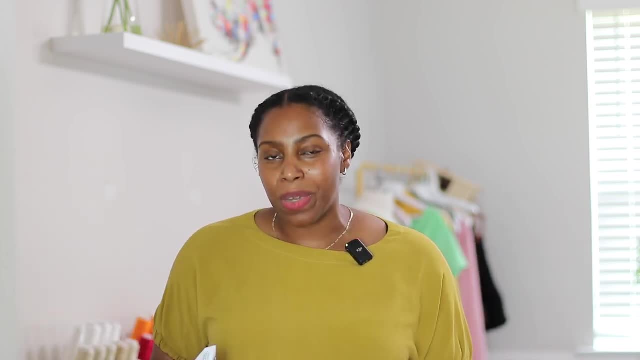 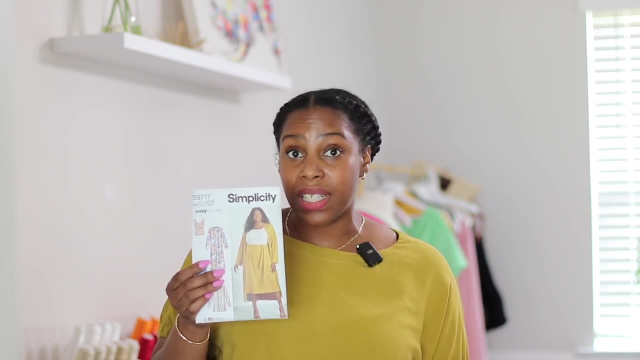 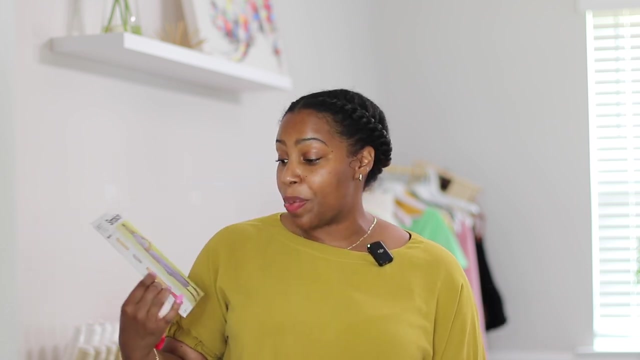 you can listen to people and take their opinions, but also do what works best for you. Okay, So again Simplicity 9717,. I think it's a great pattern, And again it is available in the Mrs Sizes as well. Next pattern up this is Simplicity 9757, another easy to sew pattern. 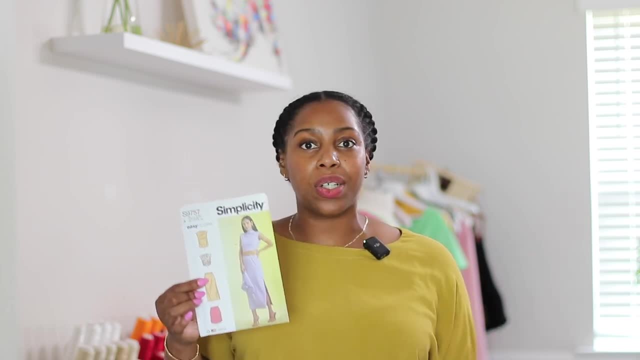 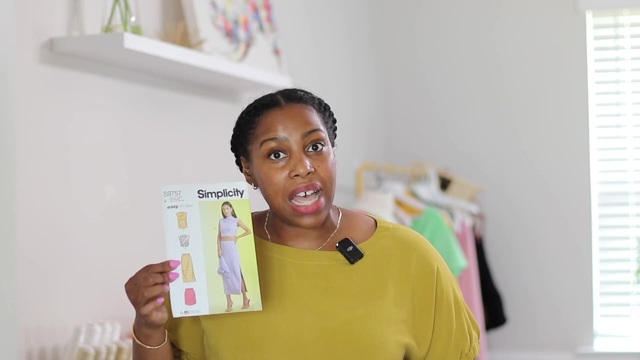 I think this one is really cute. It's really trendy. If you are into kind of crop tops and skirts, I think this is a great one to try out. What I like about this skirt on Vue D is that it has some ruching on the side, So that may be a great way to try it out. And if you're looking for a 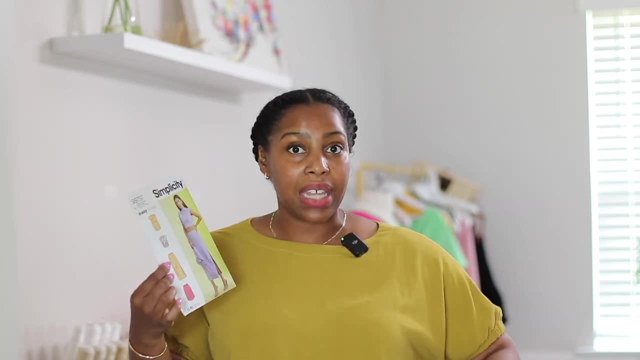 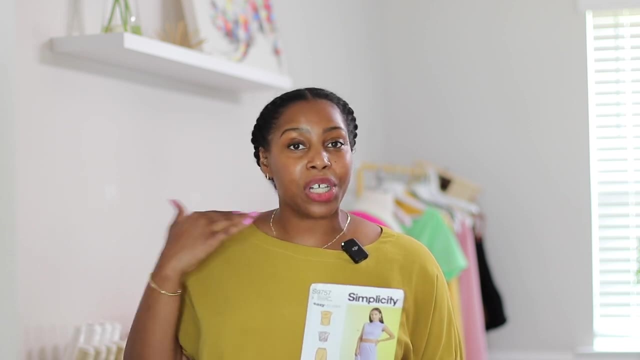 technique for an advanced beginner. even on Vue B it has the ruching on the side and that mock neck. That's something that's good to learn because you need to learn how to cut into curves so that everything lays nice and flat. So those are just good little techniques and things to 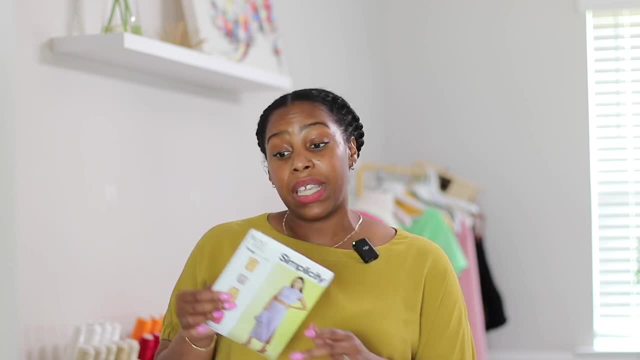 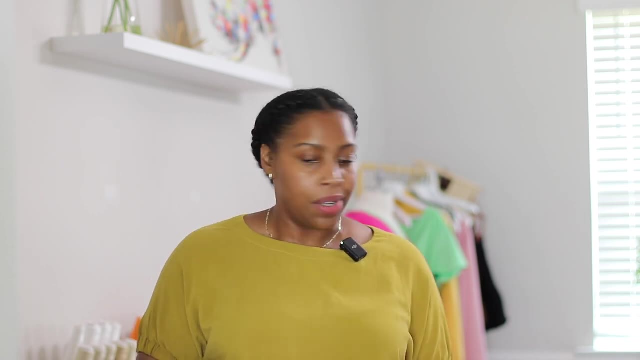 learn as you're sewing, So I do think this pattern is great for beginners. Again, it's just an easy pattern. It is a knit top skirt and it's in two lengths. I feel like a lot of these projects are knit. I may have to do one for woven then, because this is very knit heavy. 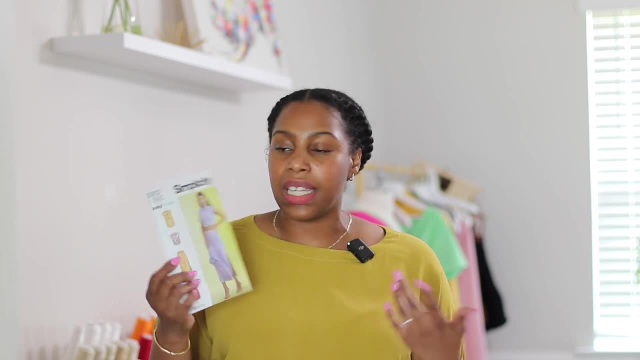 But yeah, I think this is really great. I think it's perfect for the season. I think this is one of their summer patterns, So I really do like that. Let me pull out the guide so we can just look here. You have nine pattern pieces in here. Again, I think that's great for a beginner or an. 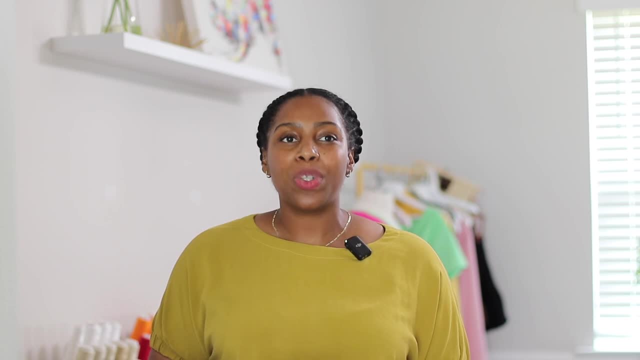 advanced beginner, You'll be able to kind of get through the project. I won't say quickly, because I'm not all about fast sewing and getting things done fast, but it's not something that's going to take you a week to sew. I feel like you can probably get through it, depending on your schedule. 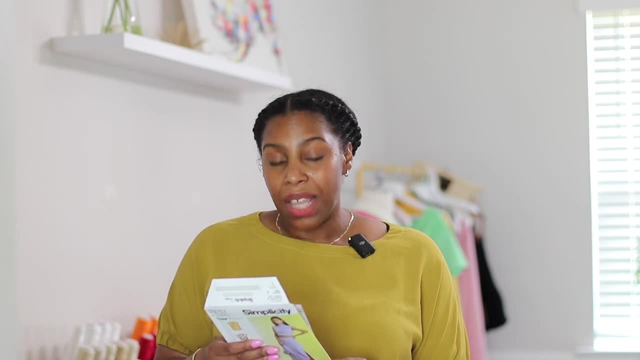 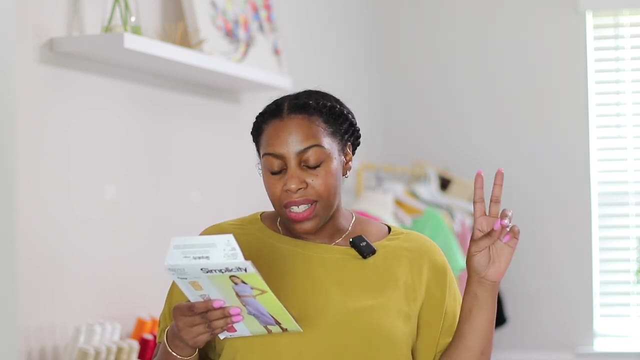 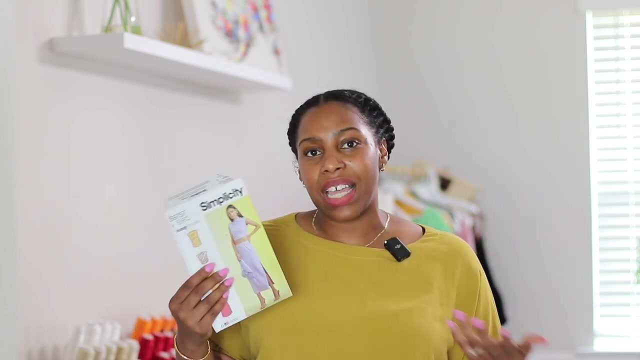 Two days, three days at max, But it shouldn't take you a week, not unless you're just super, super busy. But for view A, it's two pieces. For view B, it's two pieces. You literally have the front and back. So it's really. these are great projects, I think, to sew And, like I said once, 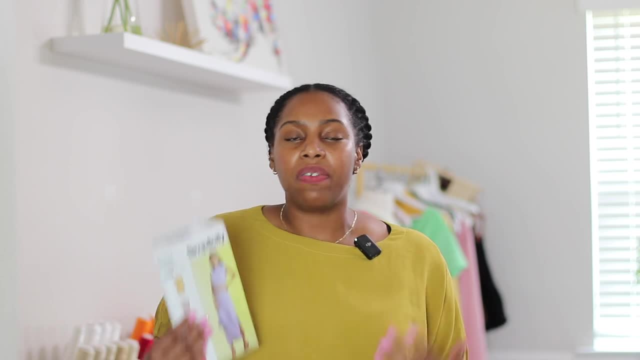 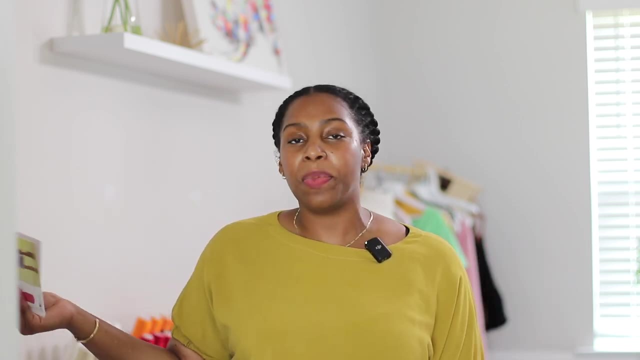 you start sewing easy projects. you just get more confident in yourself, more confident in your skills, and that's where the growth happens. So it's okay to start with projects that just have two pattern pieces. Go for it, Make 10 of them. 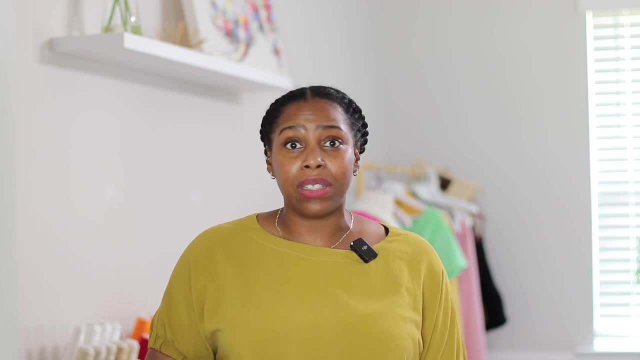 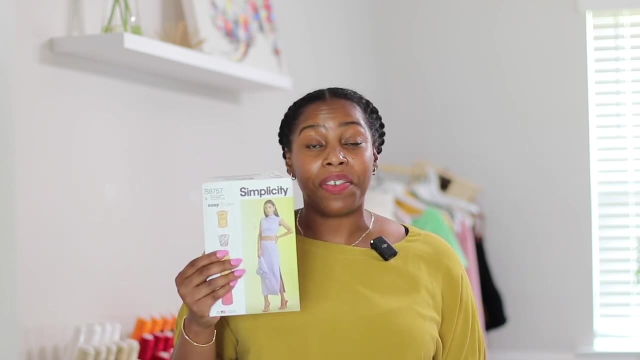 I guarantee you the 10th one is going to be better than the first one. So no one's judging, At least I'm not. anyway, No one's judging. Okay, So again, simplicity, 9-7-5-7.. 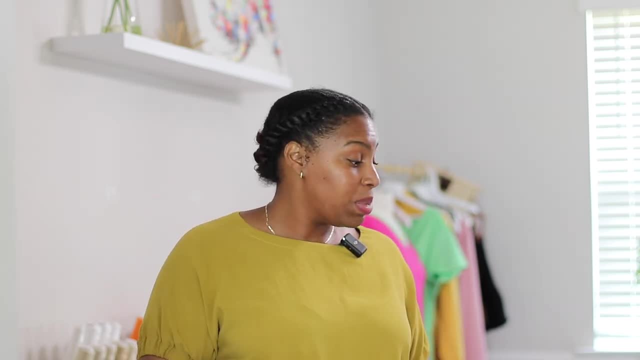 Pattern number four in my five patterns is simplicity 9-7-5-1 and simplicity 9-7-5-2.. I may need to make another video. I feel like all these were simplicity. They were simplicity. I like this because these actually say one hour. These are one. 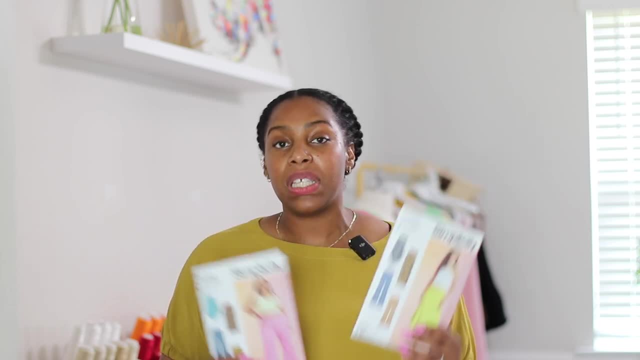 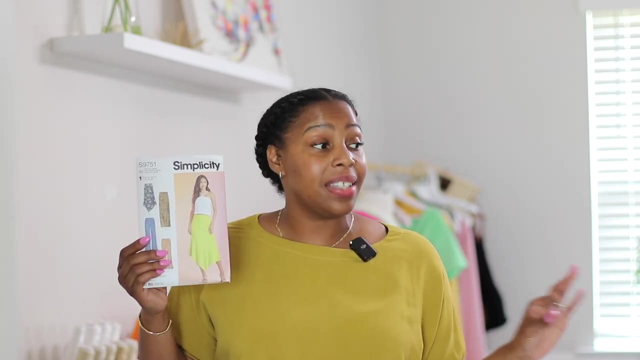 of my favorite projects. Think these patterns. they're the same exact styles. One is just in the Mrs, The other one is in the women's. This is a knit skirt and pants in two different lengths. Listen, the knit skirts and the knit tops are very easy projects to sew with, but also a nice little. 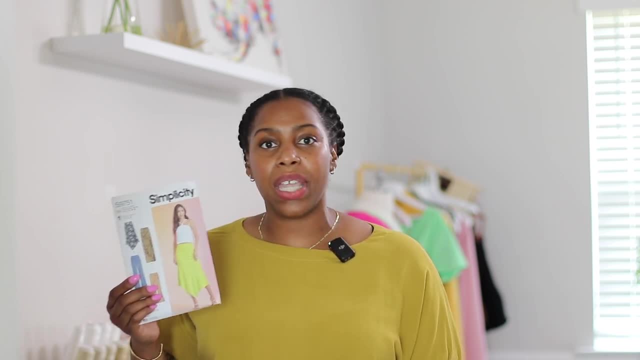 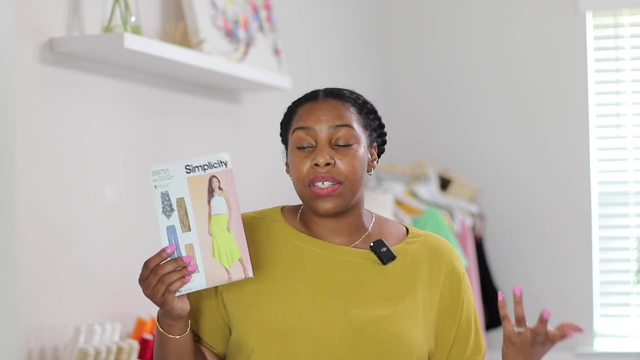 gathered skirt with elastic waistband. That's more of a kind of an advanced beginner. but you can definitely knock out some easy knit and woven projects And, yeah, like I said, just grow your confidence in it. But this again, simplicity. 9-7-5-1.. 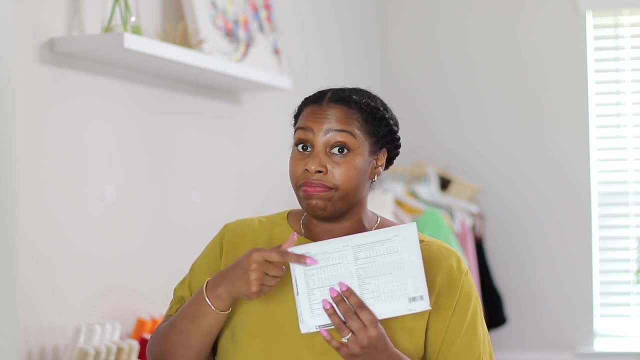 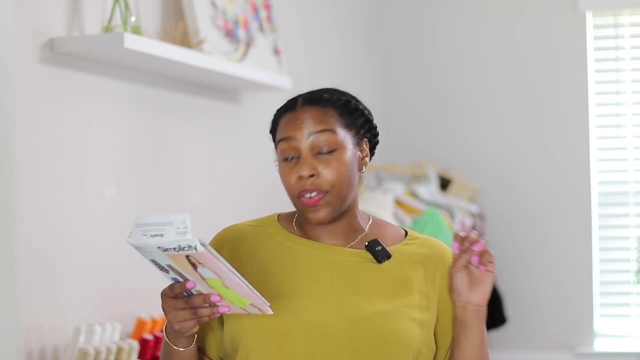 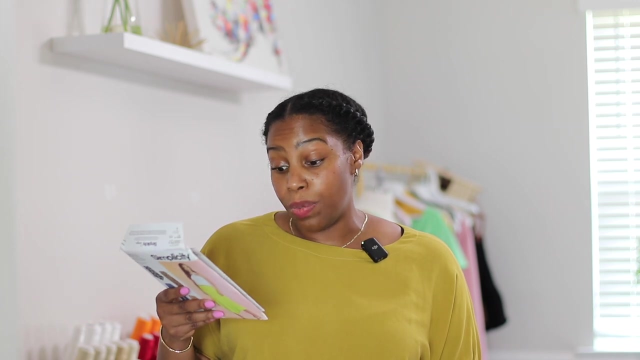 Let's pull it out. This is listed as very easy, Very easy. Let's look at the pattern. You have seven, Seven pattern pieces. For view A, you have three pattern pieces and one is including the elastic guide, So you don't even cut that out of fabric. For view B, you have two. 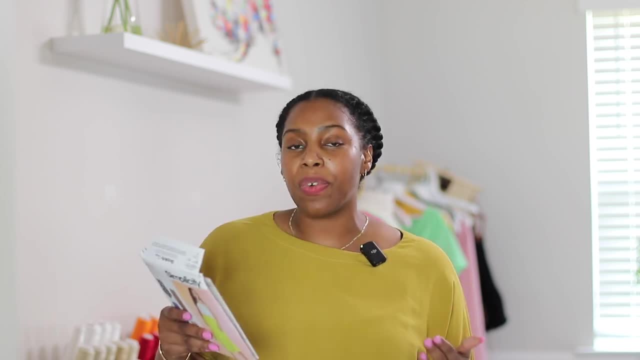 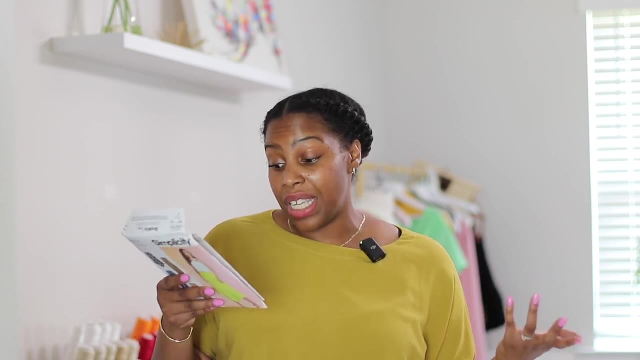 So the front and back is one pattern piece. So pattern piece number four is your front and your back. Like those. you can't go wrong with those if you're new to sewing. And then view C and D, they have four. One of them is also including the elastic guide, So very easy. 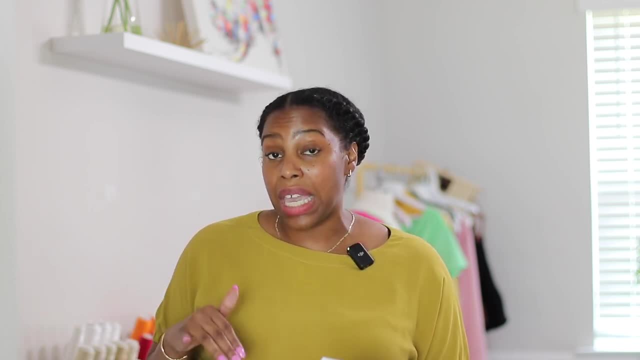 Like I said, try to keep your pattern pieces under five if you can. If you are new to sewing again, you don't want to overwhelm yourself with a bunch of pieces that you have to keep up with. Keep the pattern pieces low, sew it up, learn, grow and keep it moving. So that again is 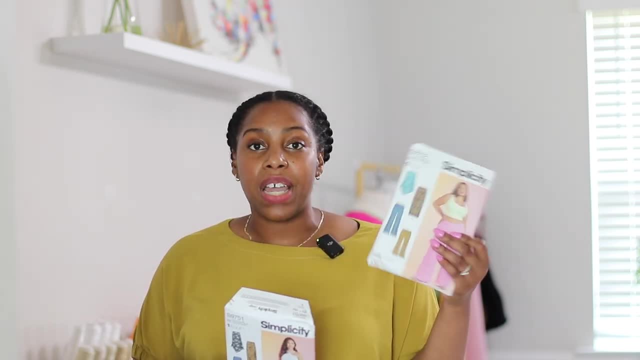 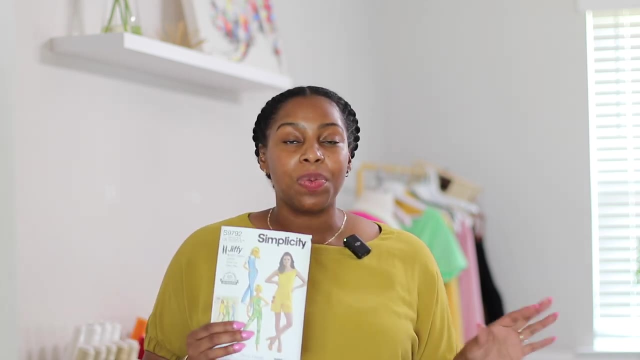 simplicity 9-7-5-1 and simplicity 9-7-5-2.. A one hour project, One hour. We love that. Okay, the last one here And this one here I've included just to kind of show you how easy these. 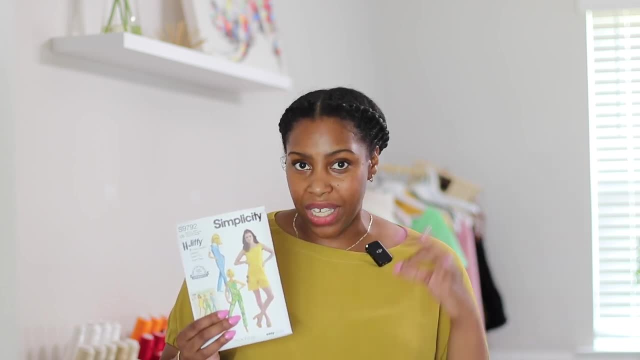 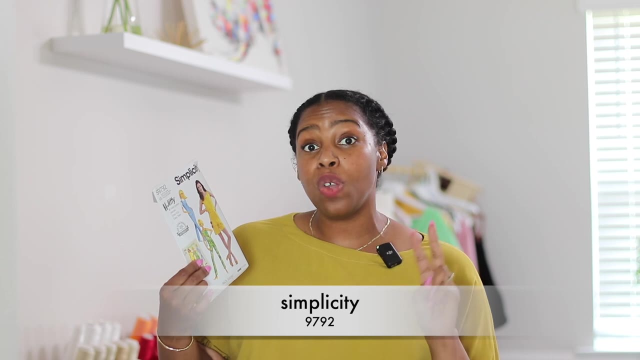 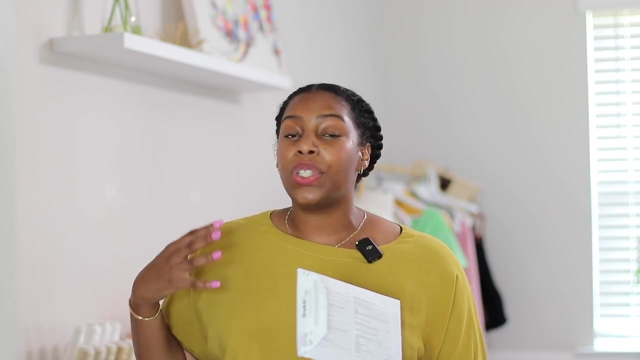 can go wrong when you are picking up patterns that say very easy, if you are completely new to sewing. So this one right here is a 1960s vintage pattern. It says that it has two main pattern pieces: easy cut, easy sew. On the back of it it's also listed as very easy, which is great, So you may. 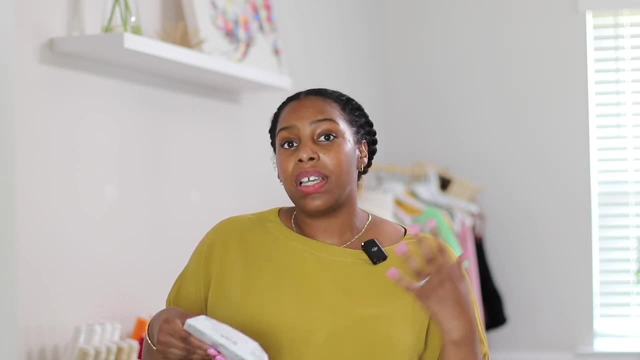 get this and go home, get ready to sew. But when it comes down to looking at the notions, if you're going to sew, you're going to have to be very careful. So if you're going to sew, you don't know how to install a zipper, that may defeat you Or you may be up for the challenge. 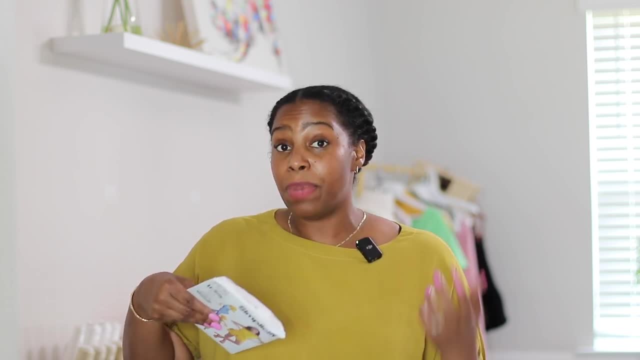 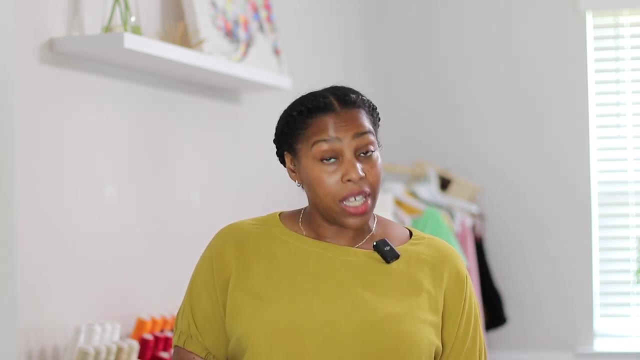 It can go either way, honestly, depending on who you are. It has buttons, It has seam binding. So these things you may or may not be ready for If you are a complete beginner, it could be overwhelming If you are an advanced beginner, ready for it. 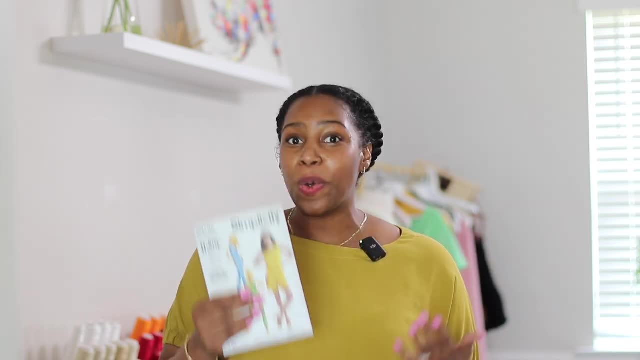 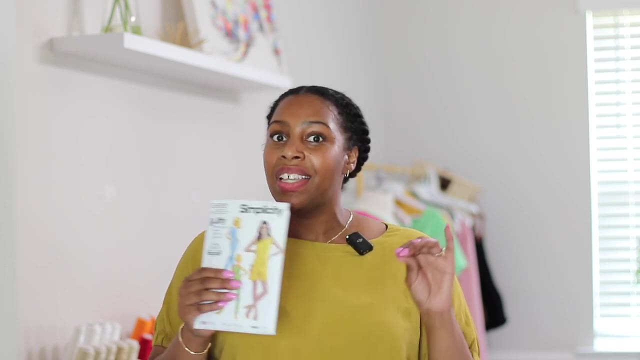 you're like, bring it on. So, like I said, it kind of depends on who you are and if you're up for the challenge or not, or if it could discourage you. So there's a couple of things just to kind of look for, to take into account. Okay, I have the guide sheet out, So let's look. 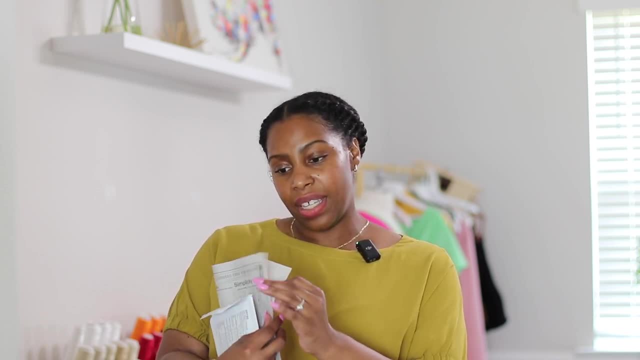 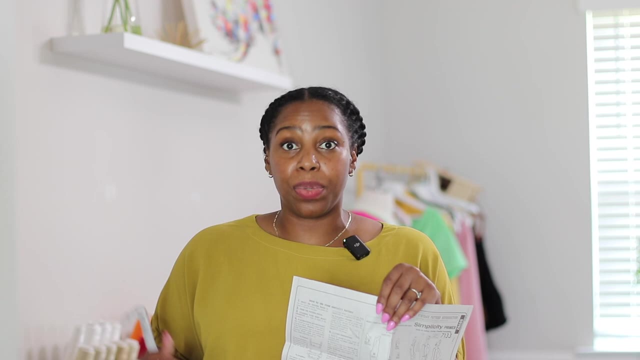 at the pattern pieces. Okay, And the vintage reproduction patterns? their cutting layout is different from what you would see in, like the ones that are just being produced today. In today's time, that's not vintage, So the wording can be a little bit different, but just keep that. 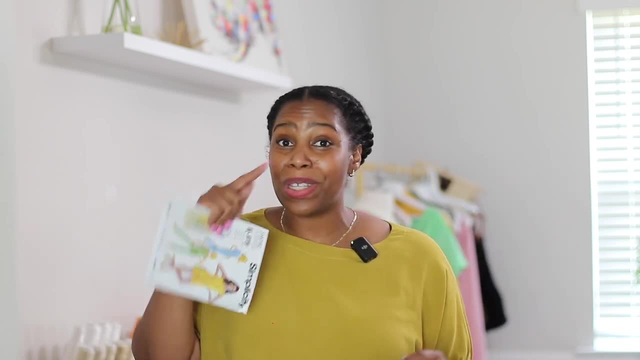 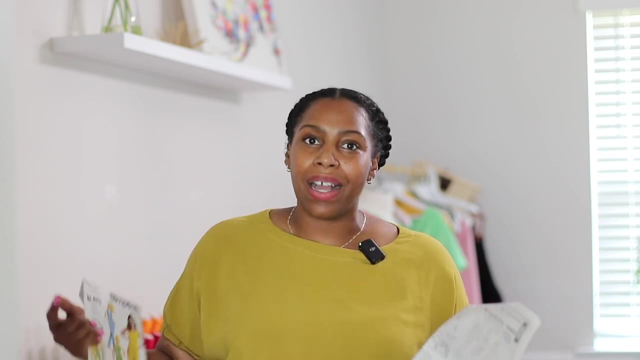 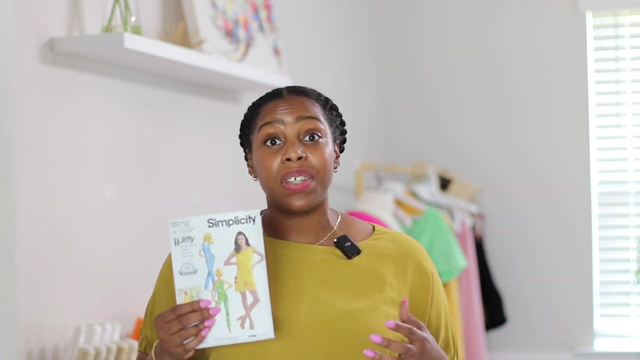 in mind, But the pattern pieces is six, So we're still right there, And one of the pattern pieces include a pocket. So I mean it's a pocket, you know. I mean it's a pattern piece nonetheless, but it's close to our five and under limit, right. So, even though this is a very easy pattern and it 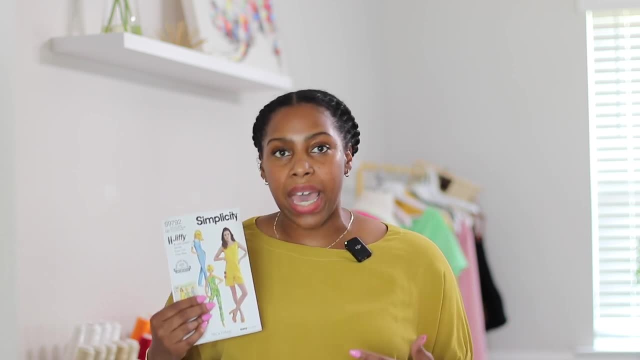 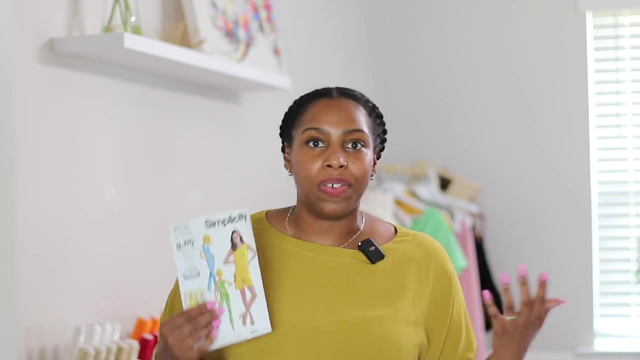 only has two main pieces, and main pieces is like front, back, yoke, sleeve, collar. those are some main pieces. You know. a pocket: you can decide if you want to add that or not. A tie belt: you may not want that, but you do need the front and the back.